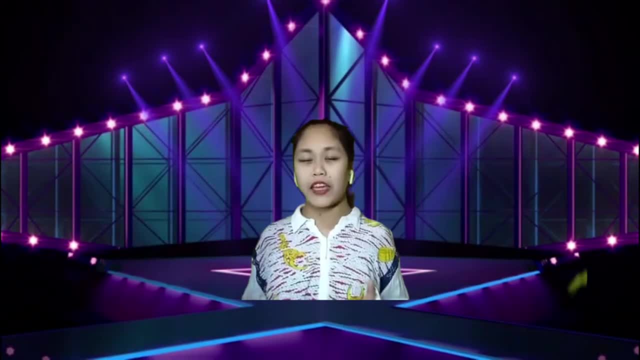 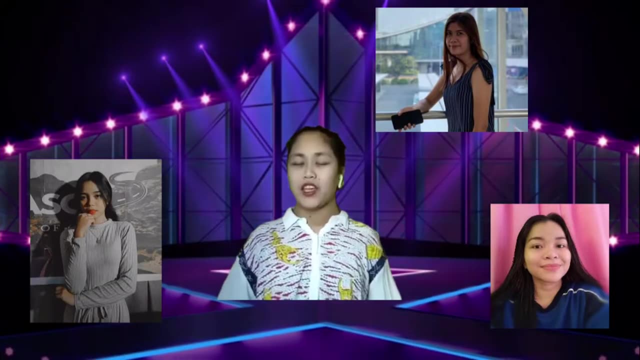 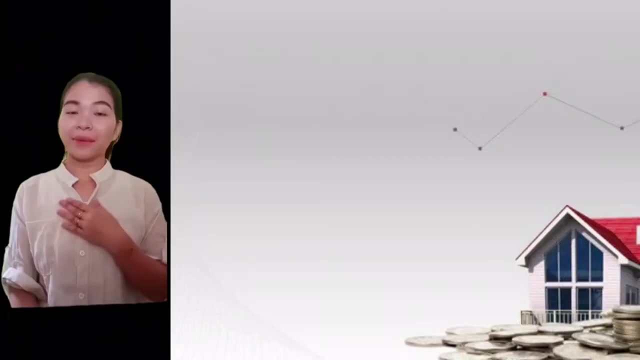 So to discuss this topic with. I have a PSA authority with me, an ecologist and a businesswoman, So, without further ado, let me invite these three with me. I am Erika Villariano, your PSA representative, And now I am going to update you about our socio-economic status here in our country. 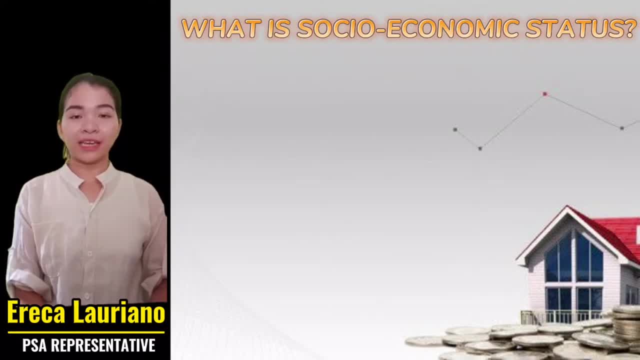 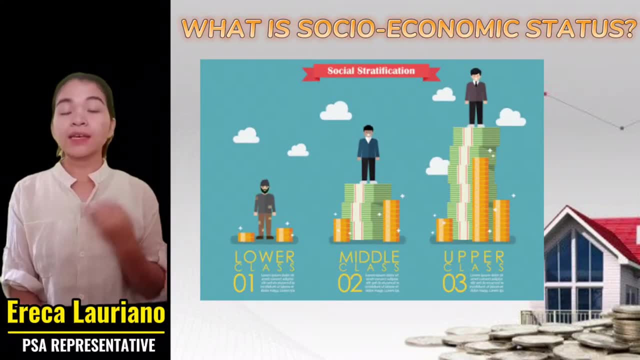 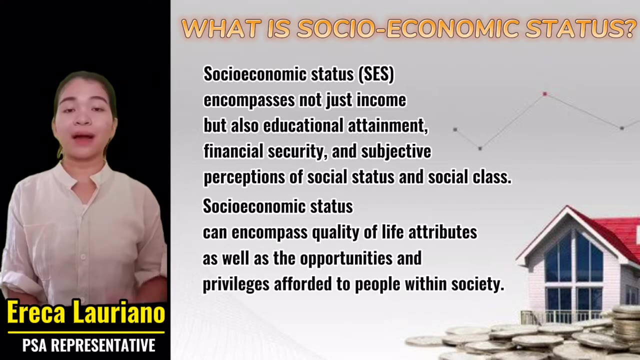 So from before we were even born, we have a designated level in the society. It's either we belong in this type of social class, it's either upper class, upper middle class, middle class and lower class, Because socio-economic status encompasses not just income but also educational attainment, financial security and subjective perception of social status and social class. 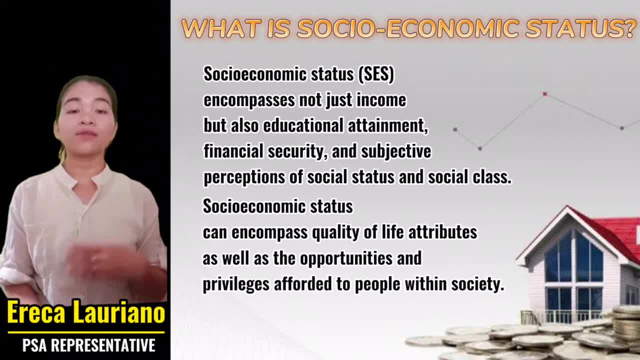 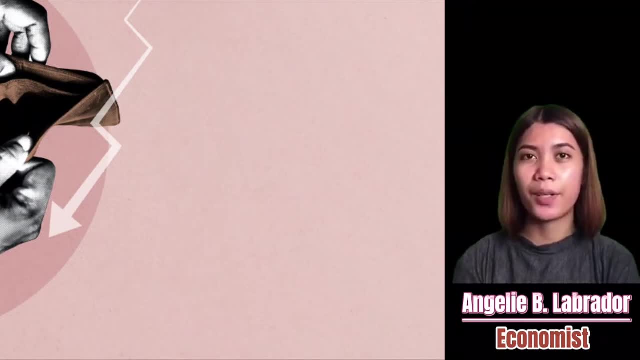 Socio-economic status can encompass the quality of life attributes as well as the opportunities And privileges afford the people we need in the society. Good day, I am Anjali Villapredor and I am going to talk about the economic status in our country, the Philippines, in accordance to socio-economic status. 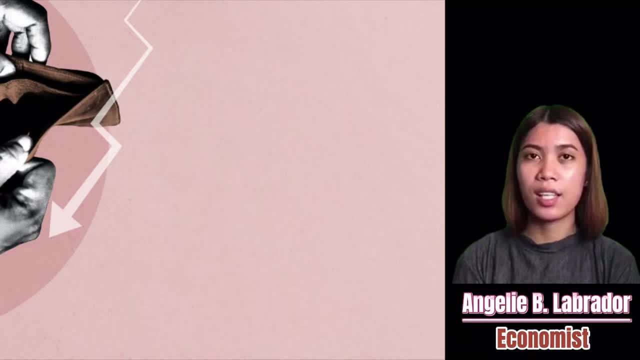 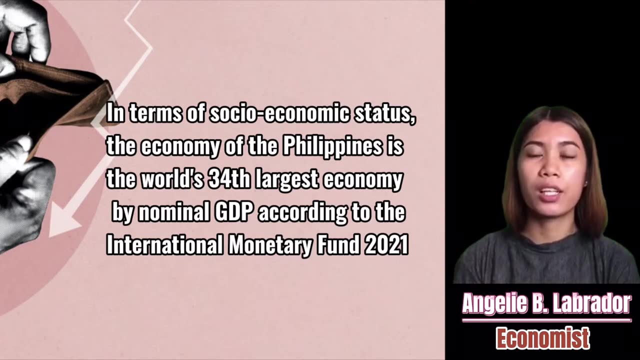 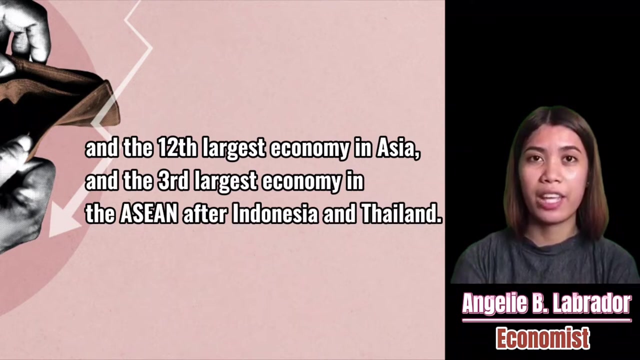 And, at the same time, the different social classes that existed in our country. So, in terms of socio-economic status, the economy of the Philippines is the world's 34th largest economy By nominal GDP, accordingly Leading to the International Monetary Fund 2021, and the 12th largest economy in Asia and the 3rd largest economy in the ASEAN, after Indonesia and Thailand. 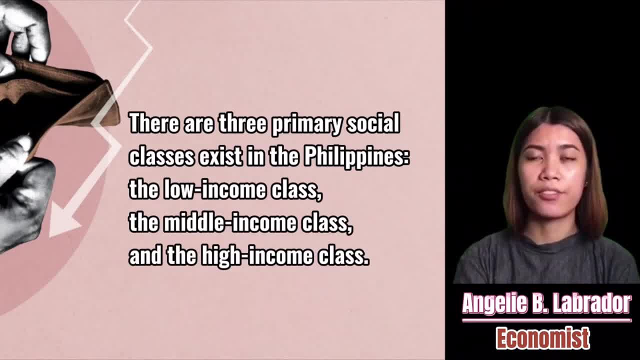 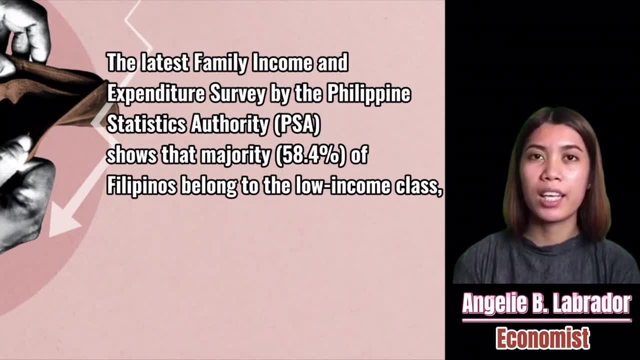 There are three primary social classes that exist in the Philippines: the low-income class, the middle-income class and the high-income class. The latest Family Income and Expenditure Survey by the Philippine Statistics Authority shows that Majority, or 58.4%, of Filipinos live in the Philippines. 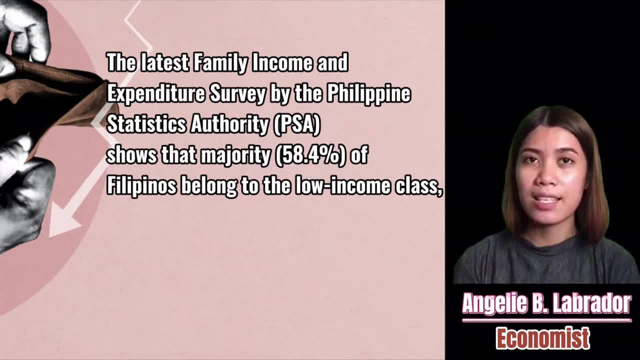 Majority, or 58.4% of Filipinos live in the Philippines. Majority, or 58.4% of Filipinos live in the Philippines. Most belong to the low-income class, while the middle class comprises around 40% of the population. 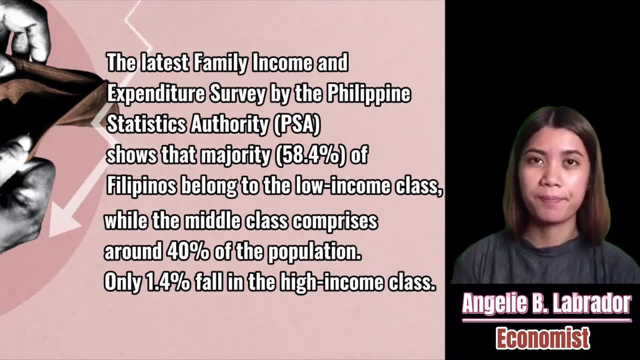 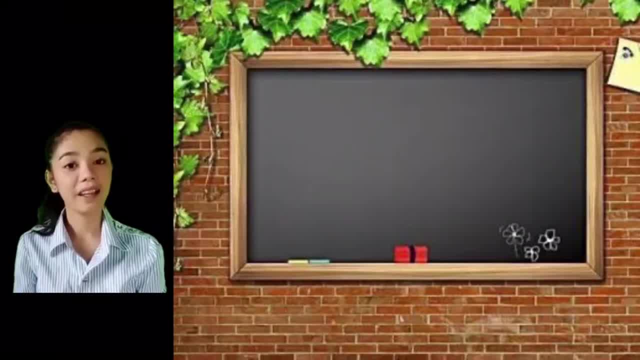 Only 1.4% fall in the high-income class. Majority- or 58.4%- of Filipinos live in the Philippines. Majority- or 58.4% of Filipinos live in the Philippines. Hi, I am Maika Lagunero.